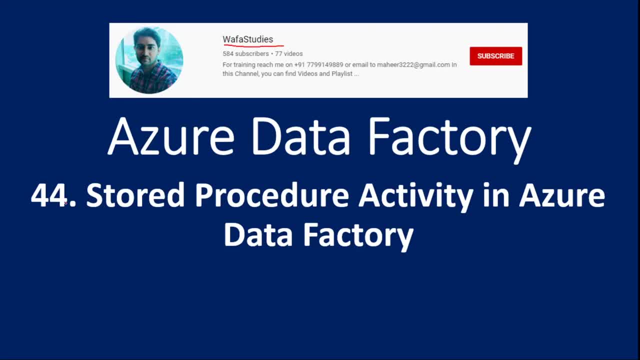 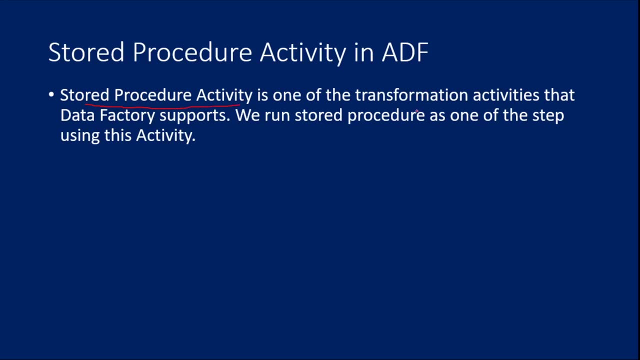 Hi friends, welcome to Wafa studies. This is part 44 in Azure Data Factory video series. In this video, we are going to discuss about stored procedure activity in Azure Data Factory. So, as we discussed from my past video, stored procedure activity is one of the transformation. 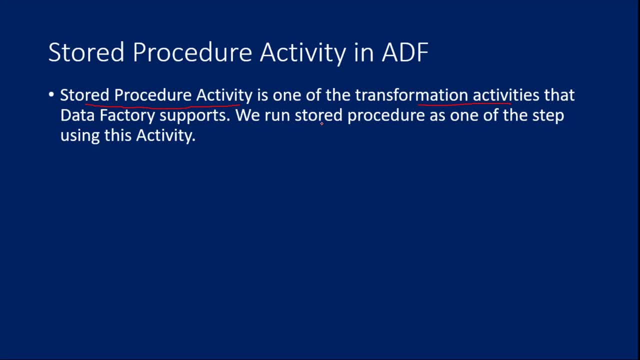 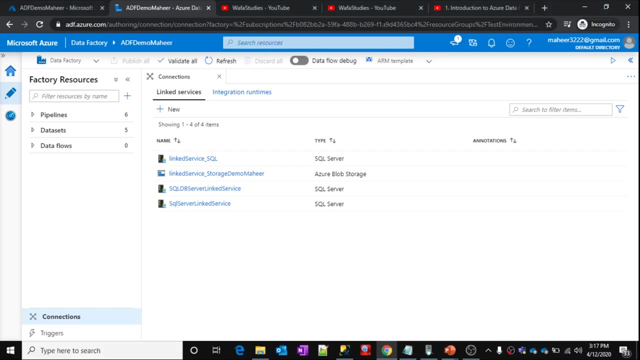 activity available inside the data factory. You can use this stored procedure activity to run any stored procedures as one of the step inside your Azure Data Factory. How to implement the same? Don't worry, we are going to look out practical implementation. now Let me go to my Azure Data Factory. This is my Azure Data Factory. Here we have all pipelines. 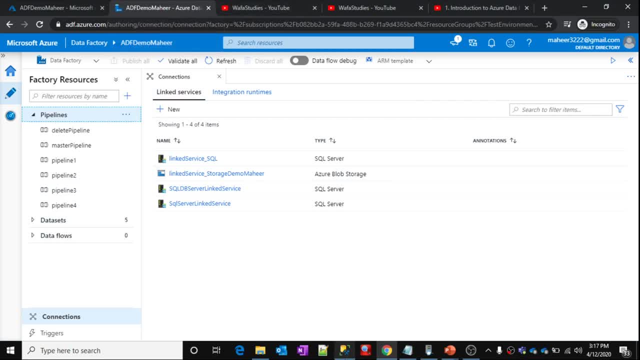 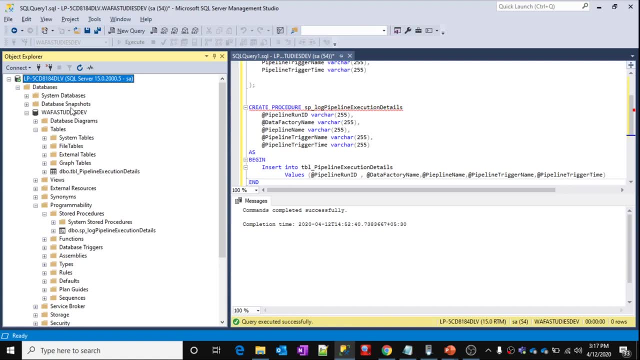 and everything. So what you need to do is the requirement is something like this: Here inside my local machine, I have a server database server- This is the one- And I have a database called Wafa studies- dev. Inside this database, I have a table called pipeline. 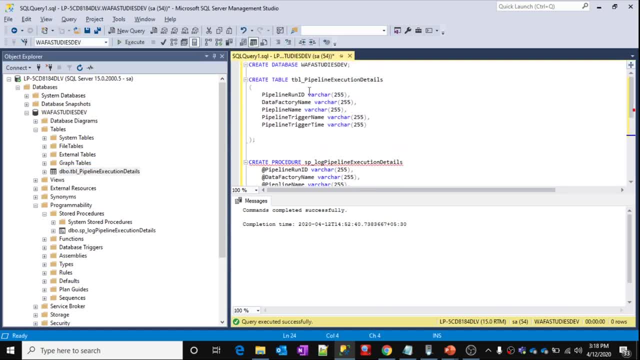 execution details. This table has few columns, as mentioned here. run ID data, factory name, pipeline name, trigger name, trigger time. Similarly, I have a stored procedure here What this stored procedure will do. this will take all these values as input parameters. 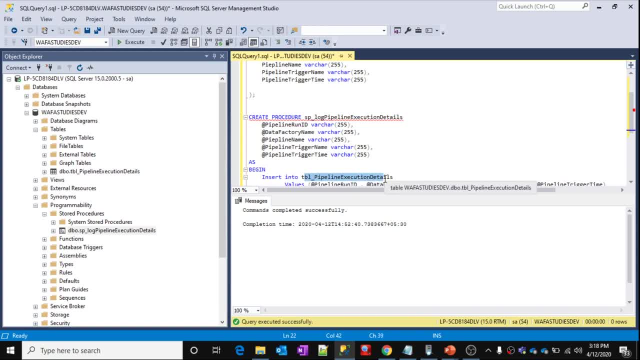 and insert those values inside this table. So idea behind this stored procedure and table is to log the data factory pipeline execution details Whenever my pipeline executes: what is the run ID? What is the data factory name? What is the pipeline name? What is the trigger? 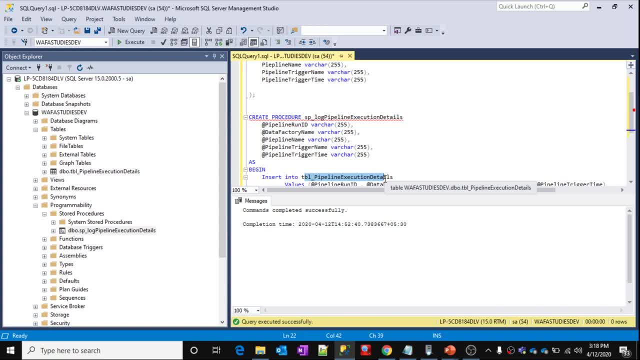 name And what is when it triggered. So all these details I want to log inside this table for my audit purpose. Okay, So I want to accomplish this requirement. So the first thing is you can achieve this requirement using stored procedure activities. That is fine. The first thing is you should. 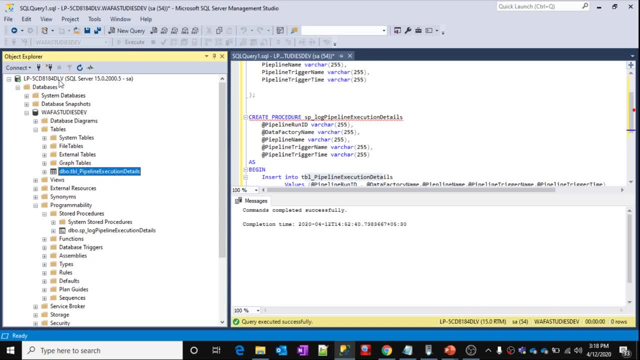 create a linked service for your database server, right first. So, as I said, this server I have inside my local machine, that is, inside my local desktop. So this is not something Azure environment, right? This is on-premises environment. You can assume like that, right? 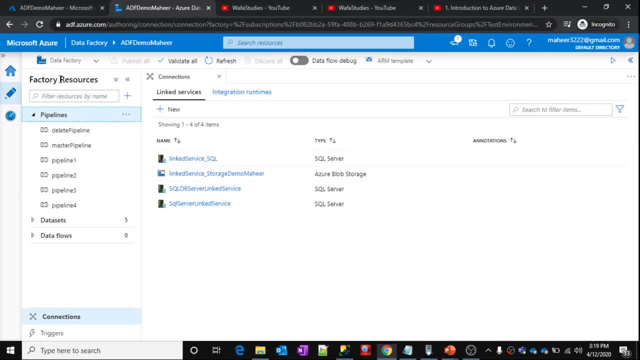 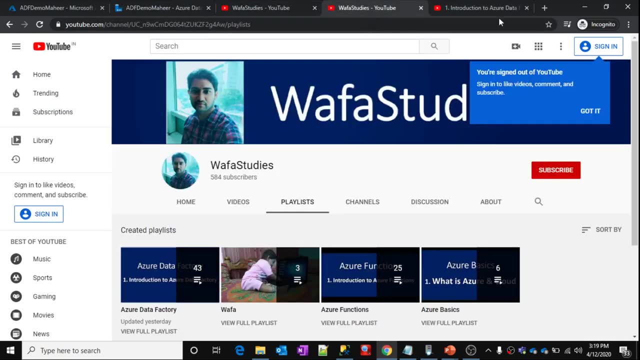 So if you remember from my past videos, let me show you that. If you go to YouTube, Wafa studies, search like Wafa studies, open my channel and go to playlist, open Azure data factory playlist. Then here, right inside this self-hosted integration, runtime and integration. 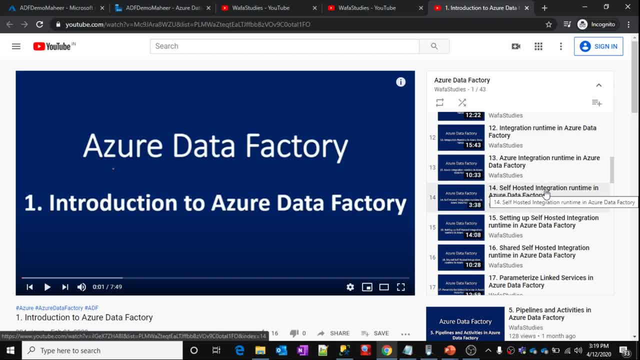 runtimes. I have discussed the difference between what is actually what is integration runtime and what is the difference between Azure type integration runtime, self-hosted integration runtime and everything. So self-hosted integration is actually which will help you to connect your data factory with on-premises resources. For example, in my case, I have 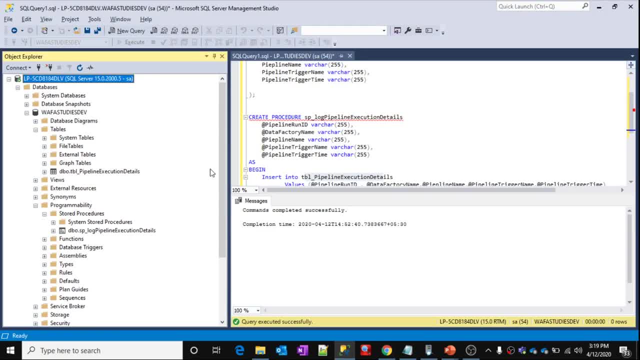 a database server Inside my premises, inside my local system. So I want my data factory able to connect this particular server. Then watch what I should have: I should have self-hosted integration runtime for that. So how to configure self-hosted integration runtime and everything I have? 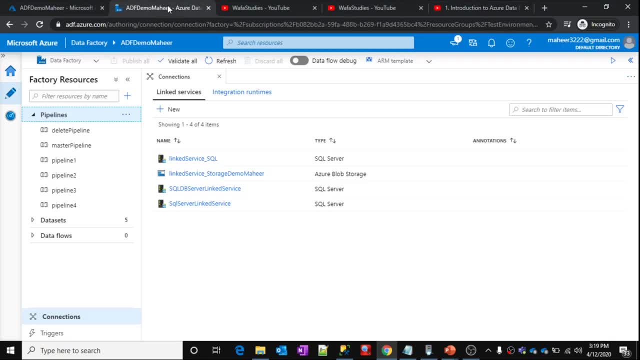 discussed here. So please watch this video, Okay. So first thing is, let's we need to create a linked service for this particular server. Okay, Let's create that. Go to link inside the go to connections, then click on this linked services. 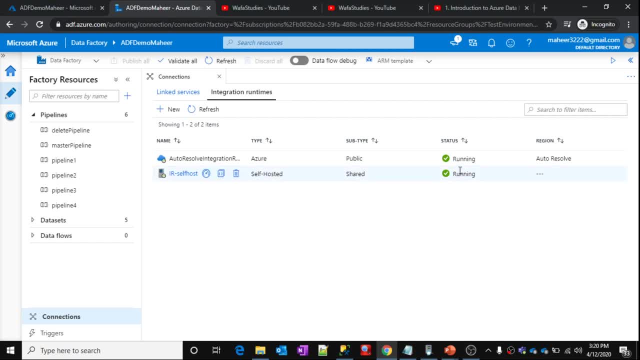 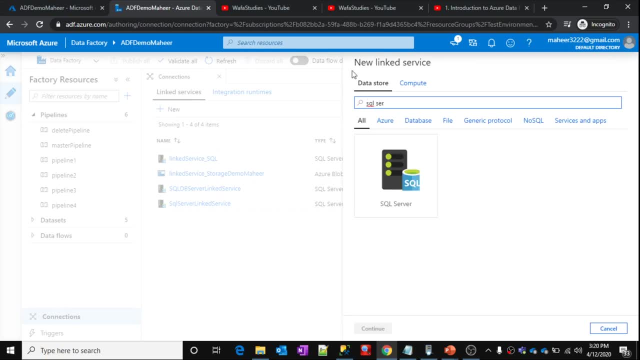 See here inside the integration and I have already created that self-hosted IR and it is in a running status, right? So let's go to linked services, click on new sign. then search like SQL server. select SQL server. click on continue. Let's give a name for your. 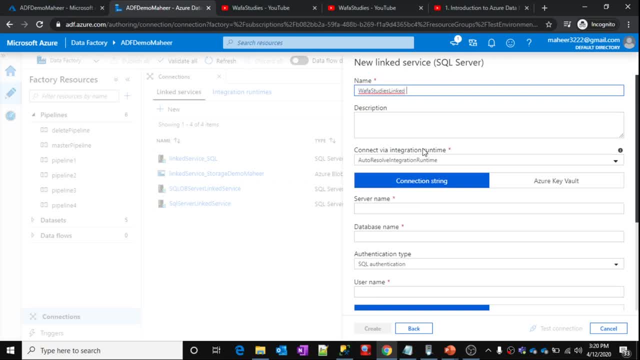 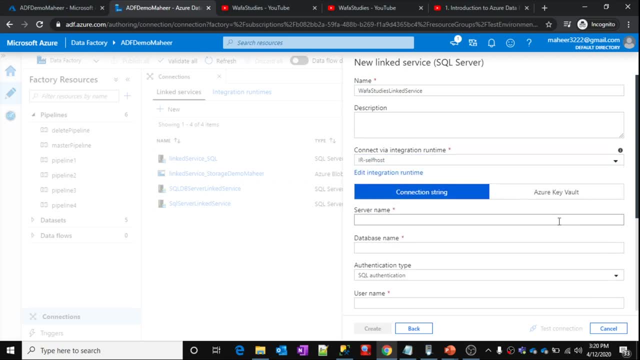 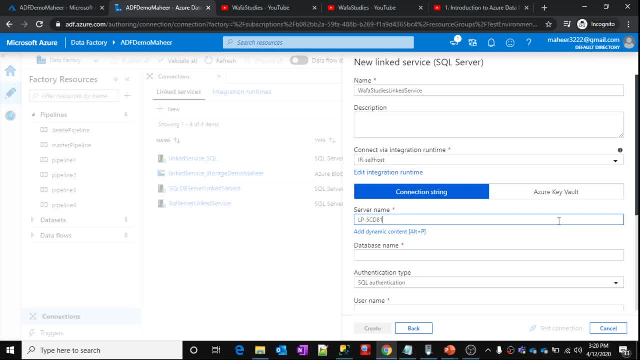 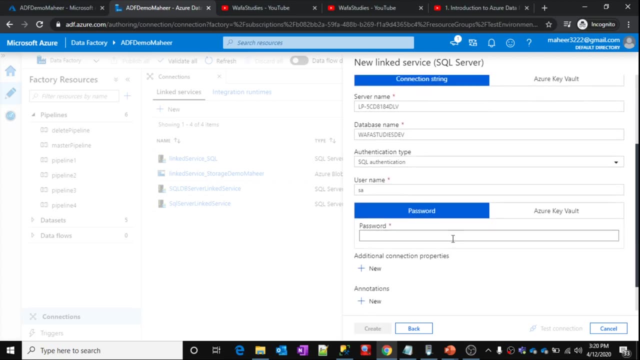 nice, Let me type it there: 818-. technically okay. Now let's give the database name Wafaa studies dev the user name. Let's type the user name. Sorry, Let me scroll down here. I need to provide a password for it. Okay, Now let's click this test connection and see. 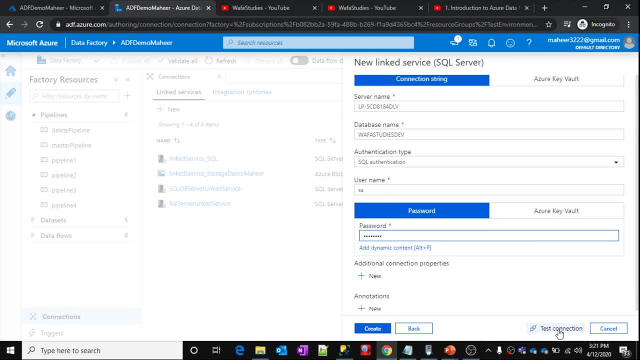 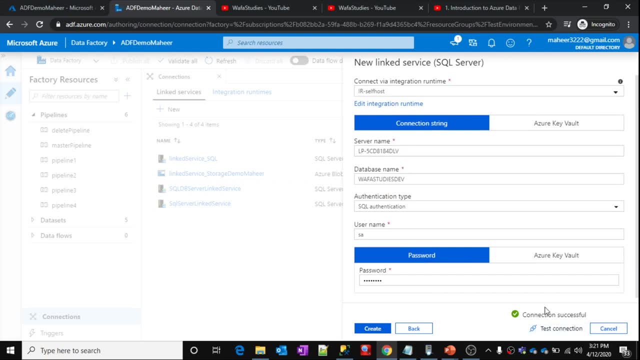 if my connection- that means if my linked service is able to connect- or not. Great, So that means you, using self hosted IR, I am able to connect to this particular server connection- is successful. Let's click on create button to create this linked service. great, our linked service. 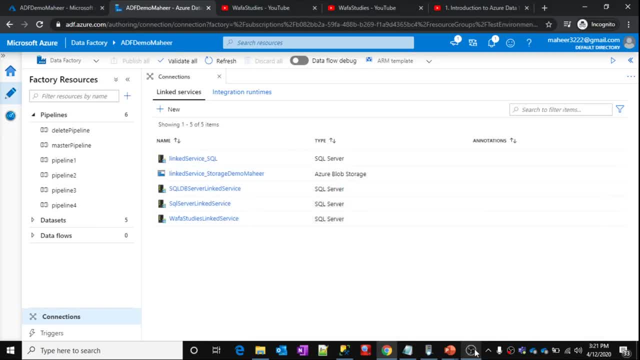 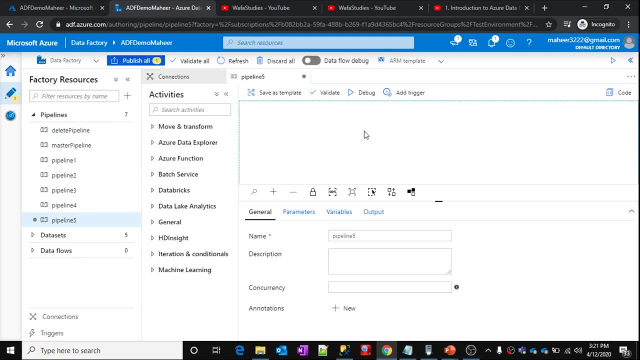 is created. you can see here. so now the next step is: let's create a new pipeline. let's assume this pipeline has so many activities. I am not going to go in details. let's assume this pipeline has lot of activities. at the end, what I want to do is I want to execute. 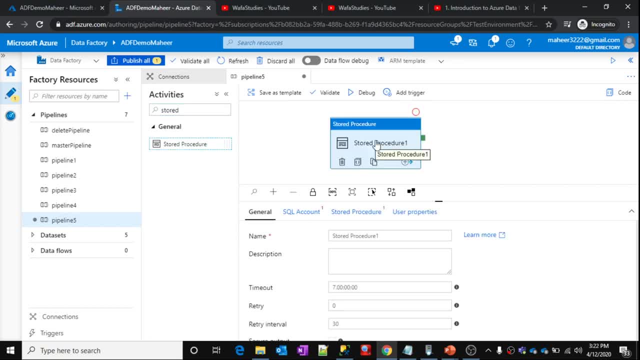 this stored procedure activity to log the pipeline execution details. okay, so once you drag and drop this stored procedure into canvas, here you can see multiple sections available to fill the configurations. so under general category you need to provide the name for your stored procedure and the description and the timeout period. what is the timeout? 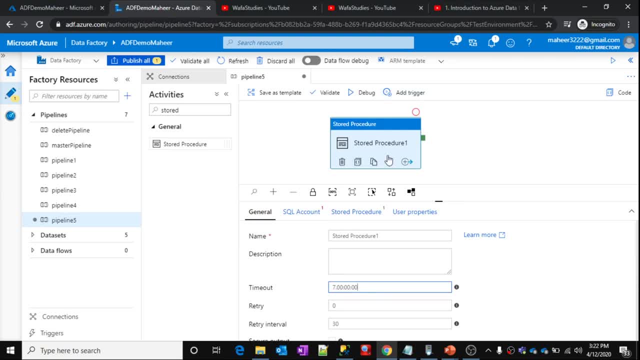 period for your activity. if within the timeout period your activity execution will not complete, then it is going to terminate the execution there, then retrace. if the activity files do you want to retry, I mean then the retry interval that means between each retry. 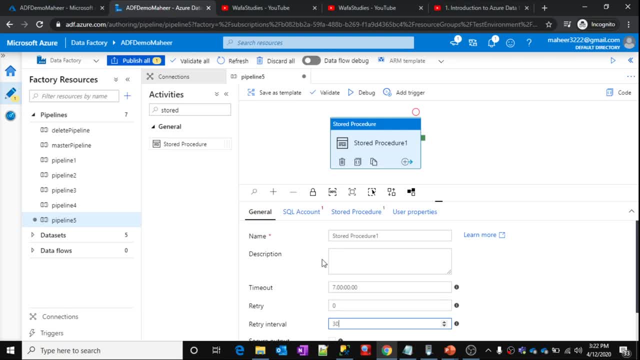 you want to maintain any gap, any interval time gap? okay, then SQL account. so here you need to select the SQL account. so I have already created the linked service for my SQL account, right? first it is linked service. you need to select that linked service here. 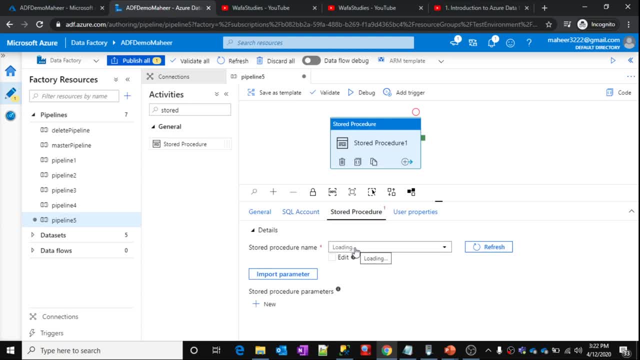 then go to stored procedure. so here, right, it will load all the stored procedures available inside your database which you configured inside this linked service. okay, So let's see once you click this dropdown. currently I have only one stored procedure. 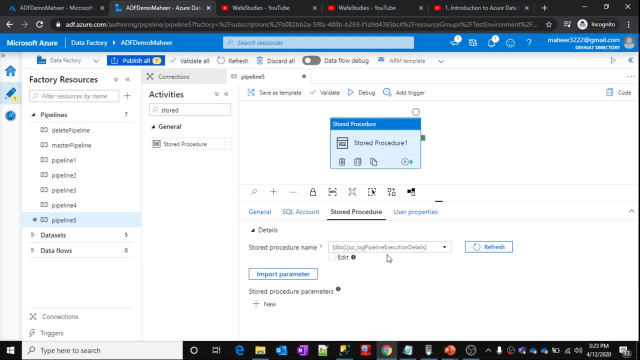 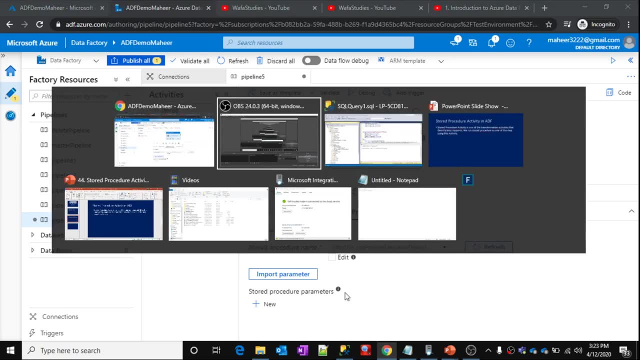 which is log pipeline execution details. so that is the reason it is showing only one, but it will list all the stored procedures. you need to pick the one according to your requirement. then the next thing is you need to see if you see here my stored procedure. 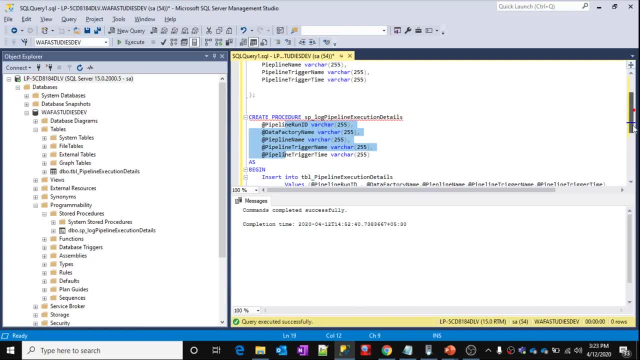 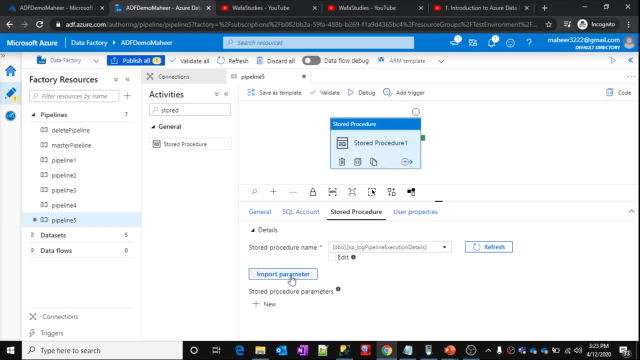 is expecting all these values as in parameters, so that these values can be inserted into the table, right? so how to pass these values? so there is something called import parameter. you can click this option, Or you can try to click this new button and by your own you can create the parameters. 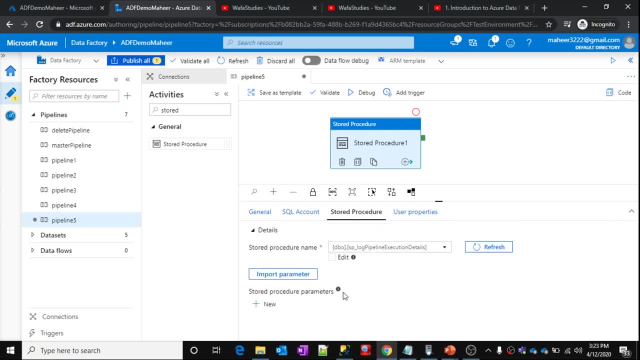 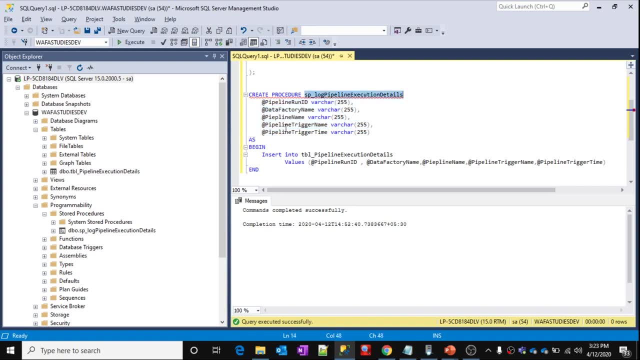 here also. so better way is click this import parameter. what it will do: it is going to look at the stored procedure which you selected and what are the parameters it is expecting, and it is automatically going to generate all these parameters there. let's see there. 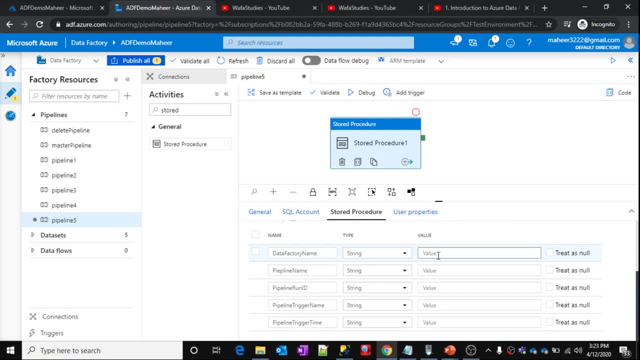 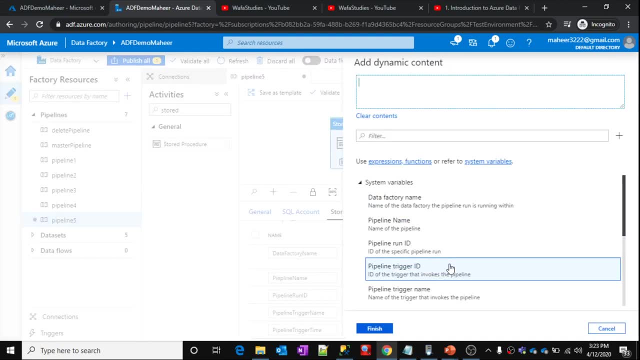 see. now all the parameters are available here. the only thing is now you need to pass the values for these parameters during the execution. so what I want to do is this is data factory name: right Click this, Then here, right all these data factory name, pipeline run id. pipeline name trigger id. 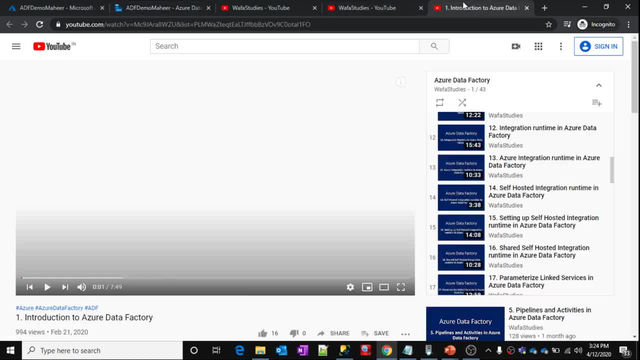 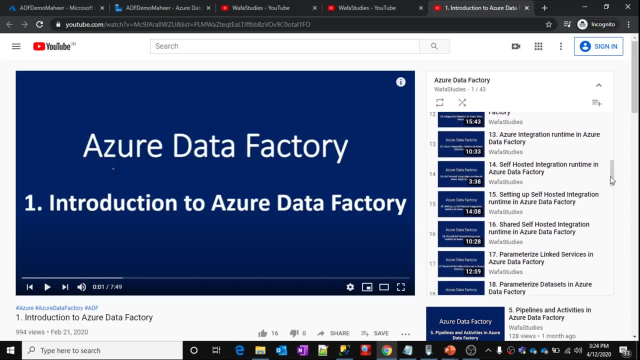 trigger name: everything are available as system variables. right, I have discussed about system variables also in my past videos, so please watch them to get a better idea about system variables. okay, somewhere I have discussed- let me see if I see here in part 20, I have discussed about system variables, so please check that. 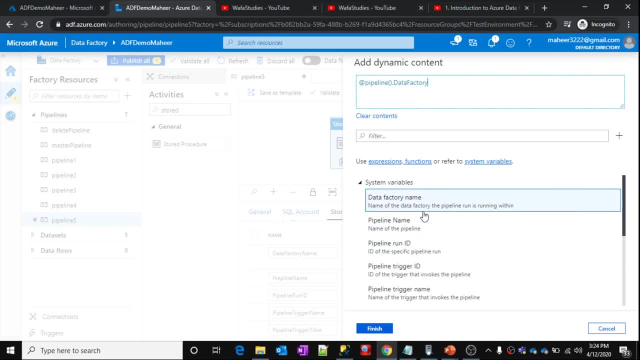 video. okay, So first thing is data factory name. let's select that, then click finish. the next value is pipeline name. Click this, Then add dynamic content. then select the pipeline name, click finish, then run id pipeline. 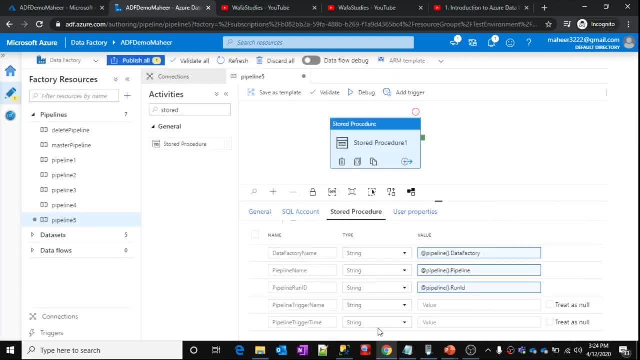 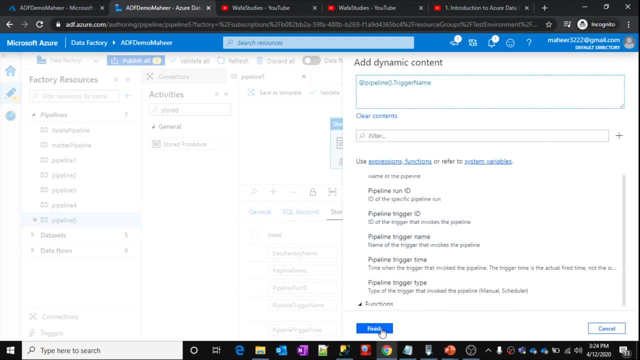 run id: click add dynamic content. pipeline run id. click finish. then trigger name. click add dynamic content, then trigger name: see here: okay, click finish. then what I want is: I want the trigger time. okay, click this, add dynamic content, trigger time: okay, which. 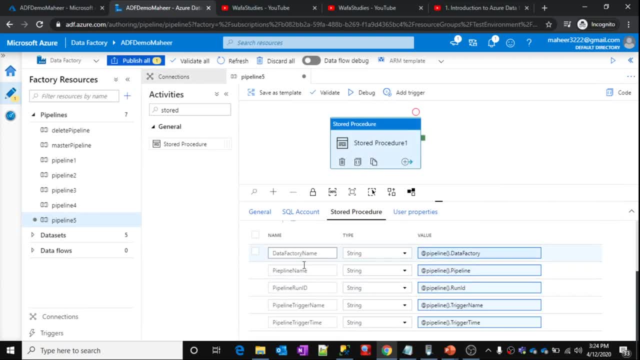 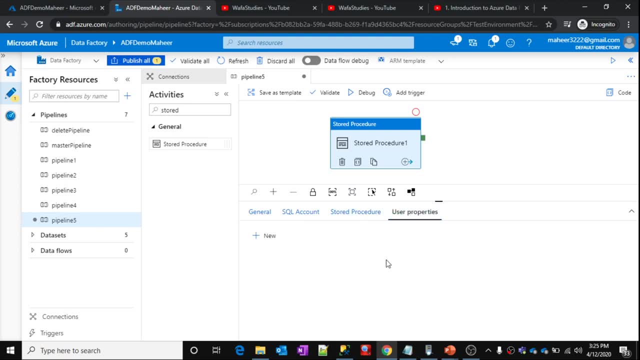 is available here. click finish so I am able to pass the values also for all my procedure parameters right. So the next section is User Properties. So what is User Properties and how these User Properties actually help you during your monitoring, when you try to monitor the activity runs. 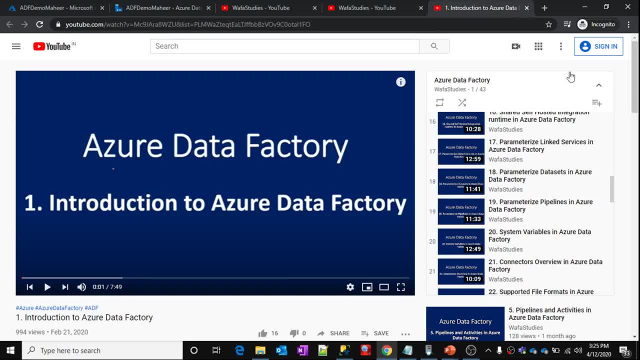 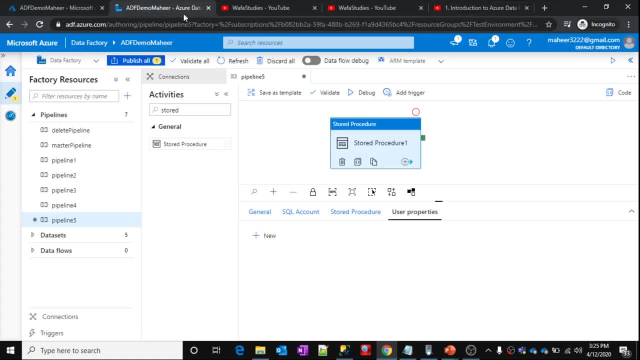 at that time these User Parameters actually help you and everything I have discussed in my past video- I think in part 30 I have discussed about User Properties. Please watch here. So that's all. actually, you will configure all these settings so that your data factory pipeline- it can go and look the stored procedure, what you want to execute. 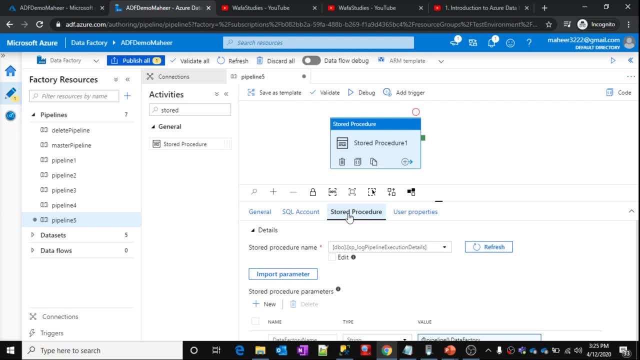 and it can execute the activity also. for you that means it can execute the stored procedure. whatever the logic you written inside the stored procedure, the logic is going to be executed automatically. So hope this given a clear idea about the stored procedure activity and how to use it. 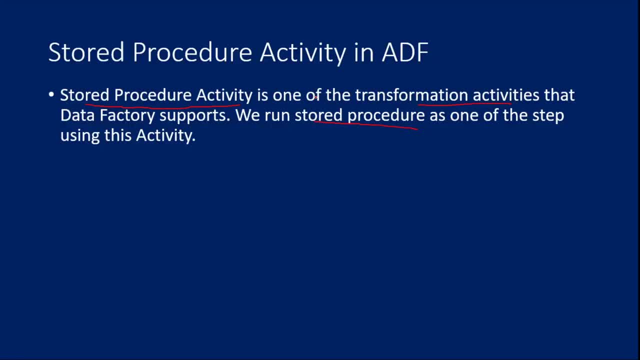 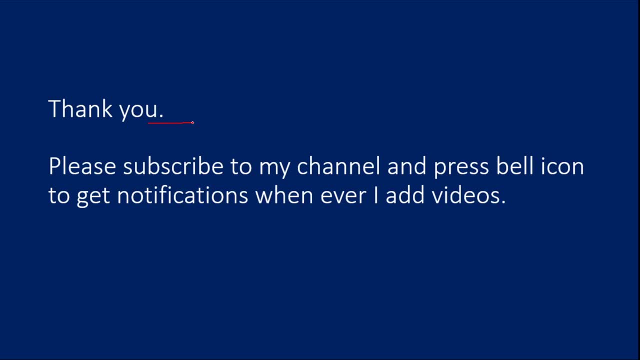 and when you can plan to use this particular activity based upon your requirement. Thank you for watching this video. Please subscribe to my channel and press bell icon to get notifications whenever I add videos. Thank you.